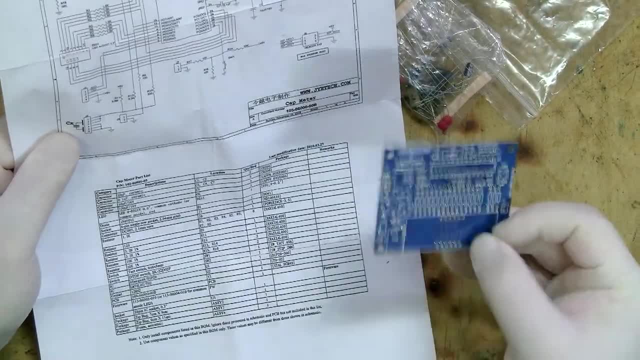 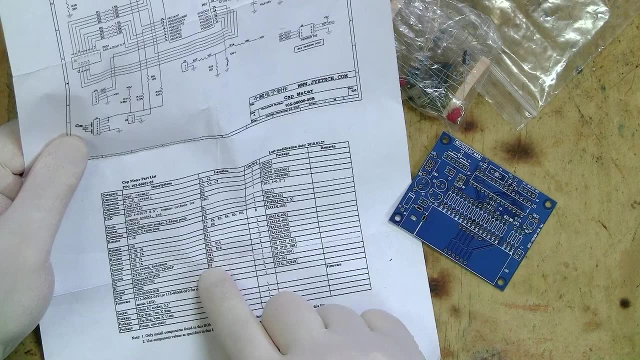 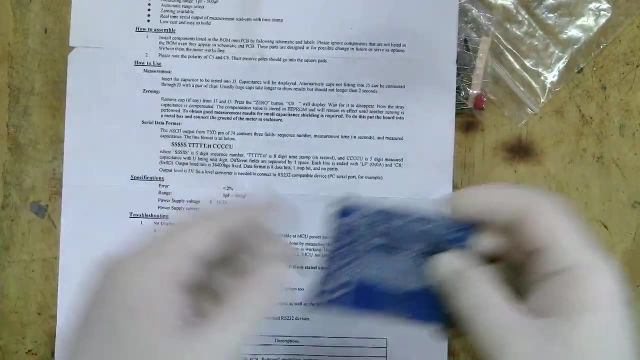 It says: this is what we need to follow. Even if there is a component that is listed on this PCB or printed circuit board, if it's not listed in the Bill of Materials, don't put it on here. So that's pretty much it. They haven't really given much information. 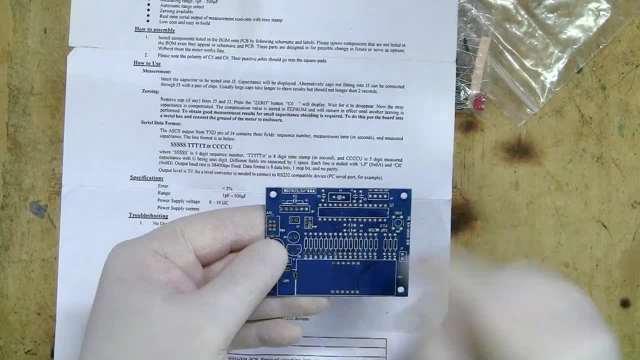 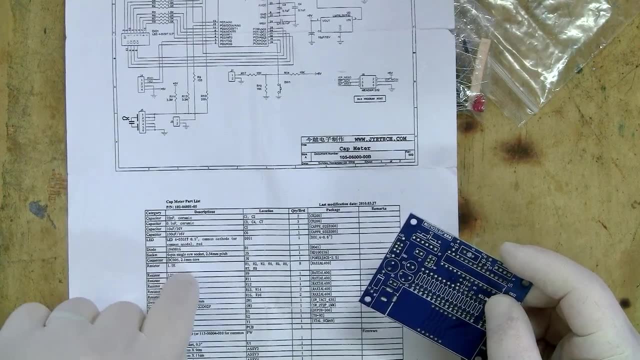 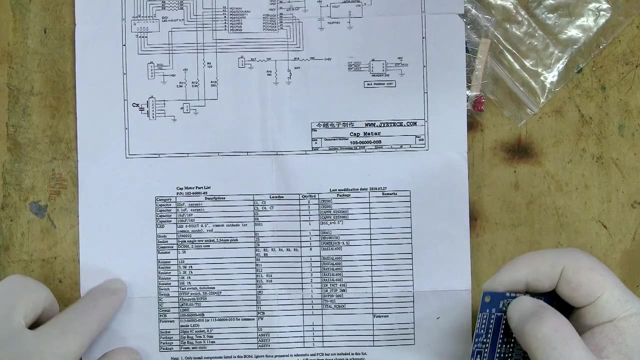 We've obviously got labels on the kit, so those labels help us work out which component on the Bill of Materials and then the Bill of Materials tells us what that component should actually be. So for example, here if we're looking at- I don't know- R12, we can look down here and see R12. 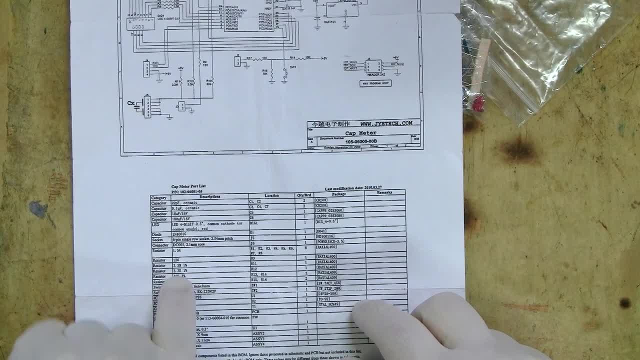 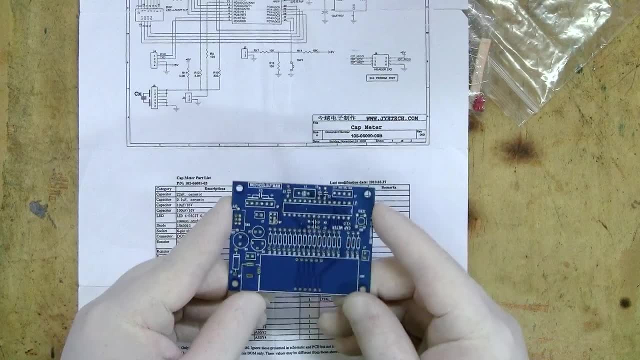 That's the location there, and it is a 3.3 kilo-ohm resistor. So that's all we really have for instructions here, But sometimes with the more basic kits you might get much more detailed instructions. They might actually go in and tell you. 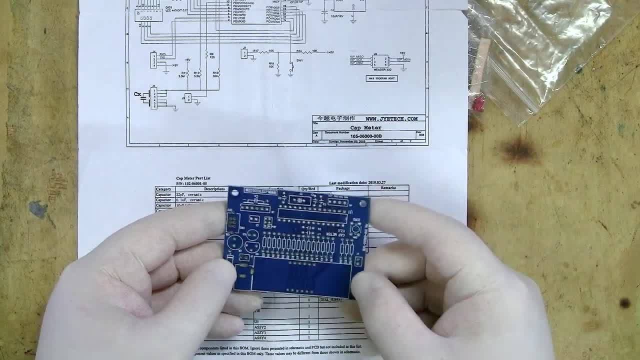 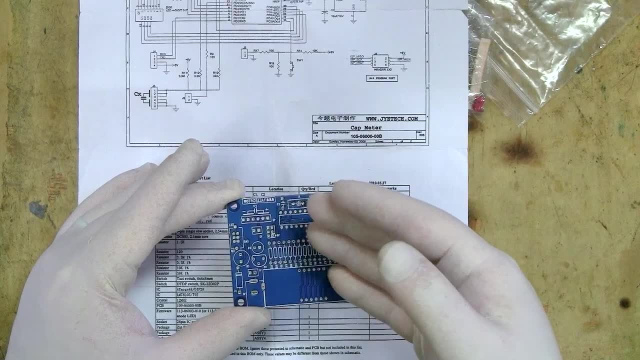 which components to put in first, which to put in second, And a lot of the time they're just doing that so that you don't end up, you know, cramming yourself into a corner. You might actually put a component in place which makes it really hard to access another component. 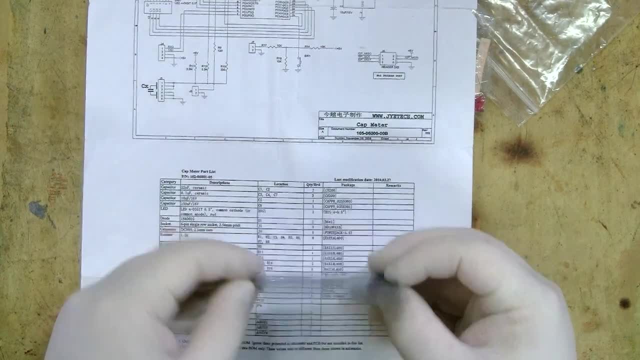 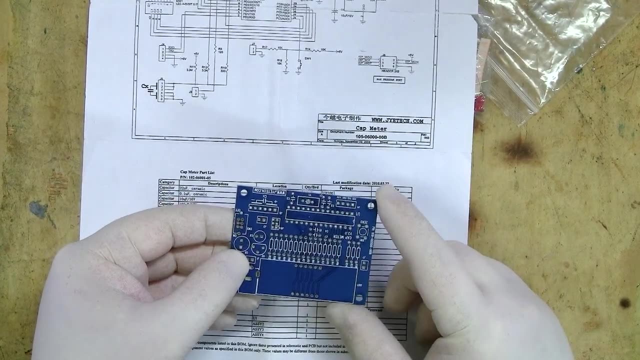 So they give you these the order in which to build it. Generally, I build these in the order of small components first and then I put larger components in later on. That's mainly because if you put big, bulky components on and then you, you know, flipping it over, 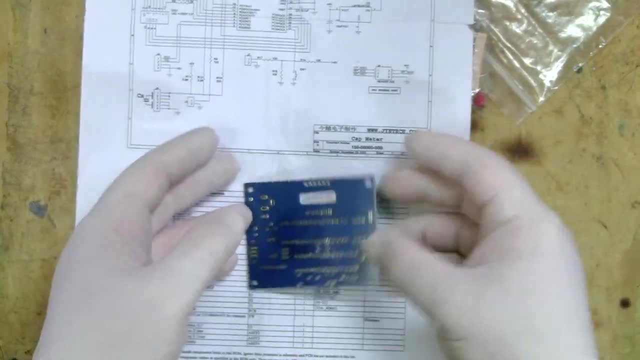 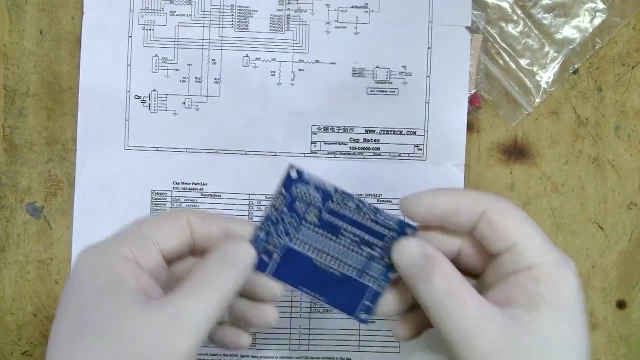 to do the soldering. you know, the board ends up rocking on the table and it gets kind of cumbersome. so I generally do all the little components and then I put all the bigger components in after that. now this is a through hole kit, so in other words it has all these holes in it. we will put the pins. 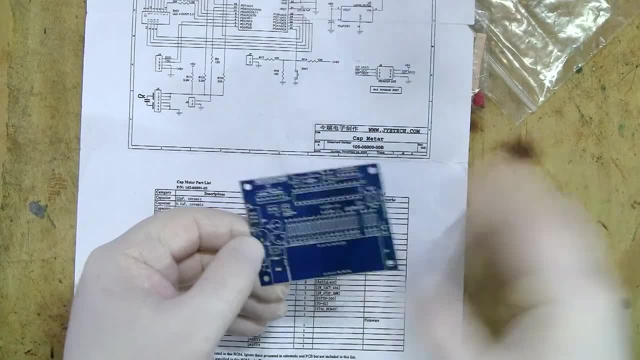 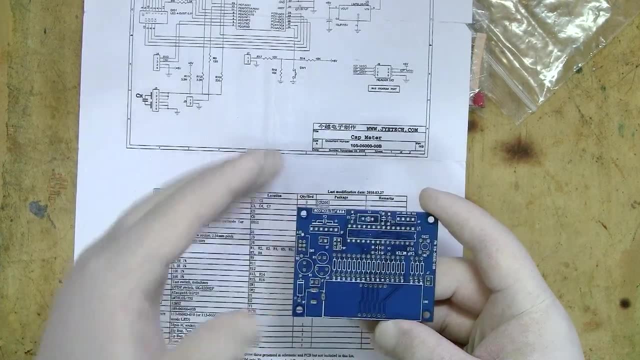 of the components through those holes and then solder them into the holes. the alternative to that would be if it was surface mount, where you just solder it onto a single side of the printed circuit board- this one. this is obviously a through hole kit and I'll be going through. 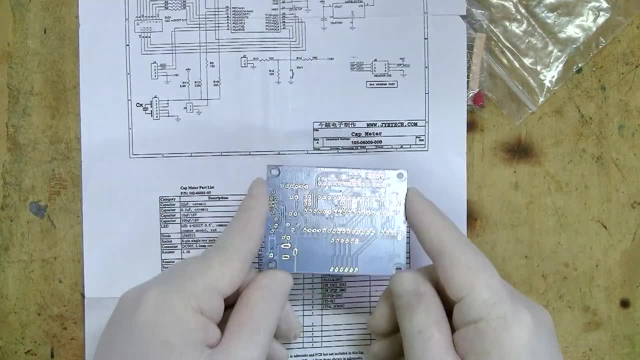 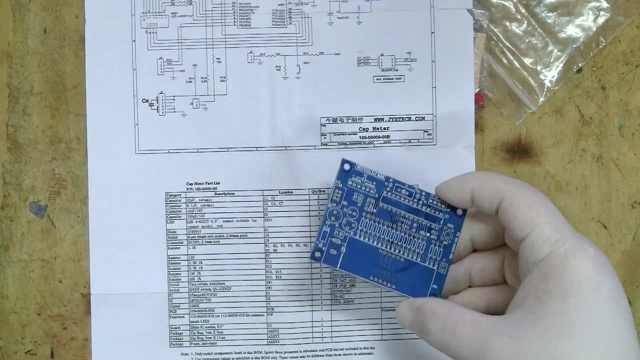 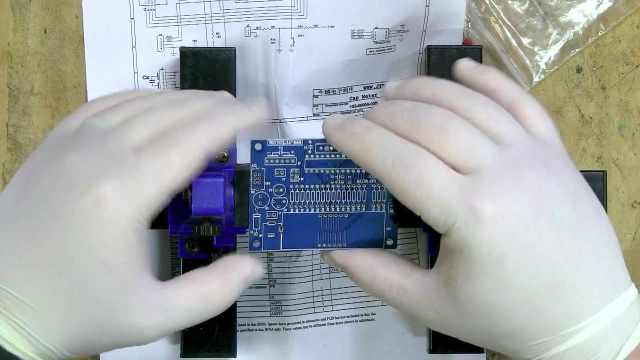 those steps. in my next video I'll be doing a surface mount soldering kit, so I'll be focusing on surface mount soldering in the next video. one of the things that I am going to use when I build this is this: it's a little stand and it allows me to get this printed circuit board and put it into. 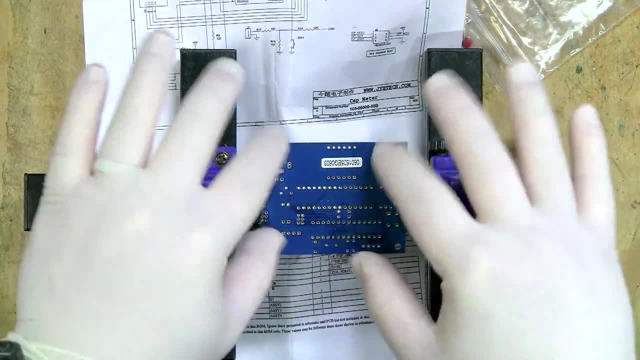 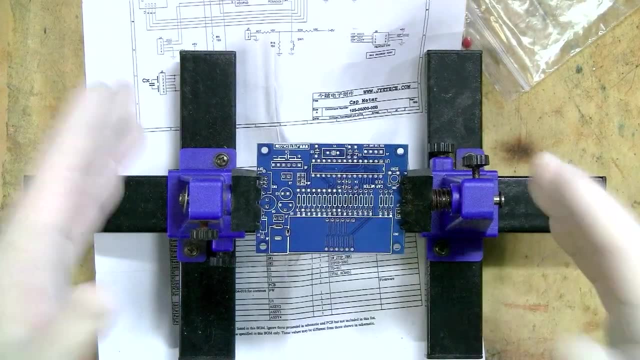 the holders, and then that gives me the ability to easily access one side of the circuit board or the other, so it holds that nice and firmly while I'm working on it. it's not essential, but it is one of the things you might want to get if you're going to do a lot of kits links in. 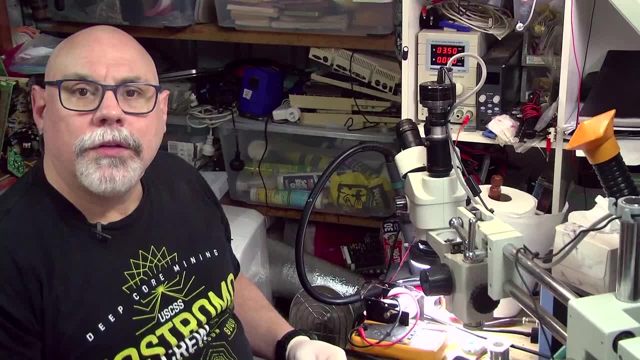 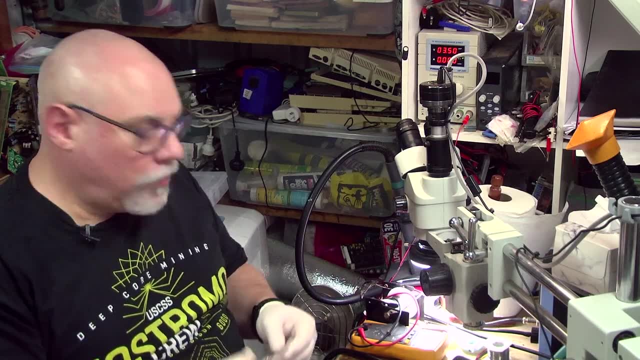 the description as to where you can buy yourself one of these stands. so this video is designed as a soldering tutorial, not as an electronics tutorial. so I'll be going over the basics that we need in order to build the kit, but I won't be going into any in-depth electronics. 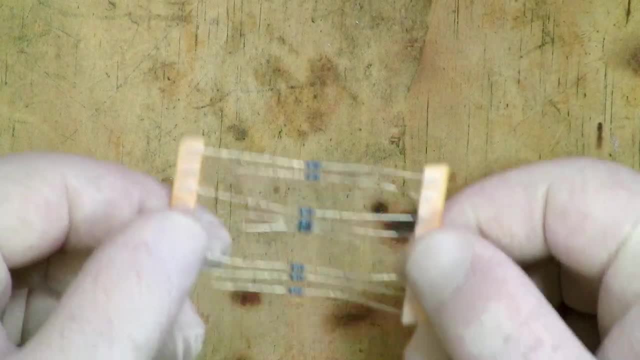 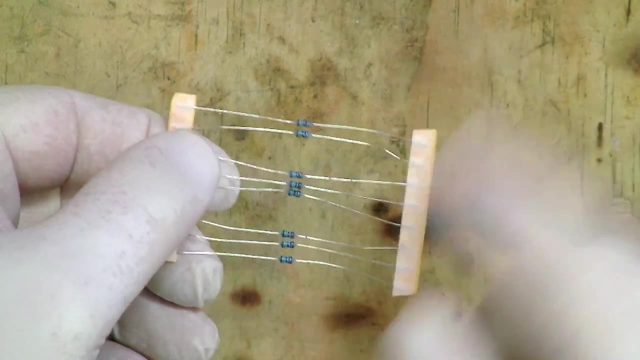 theory. the first thing I'm going to do is put all of the resistors in place. so these are the resistors here. you can see that they're blue and they have these little colored lines on them and they indicate what the resistance is. there are quite a lot of people that memorize. 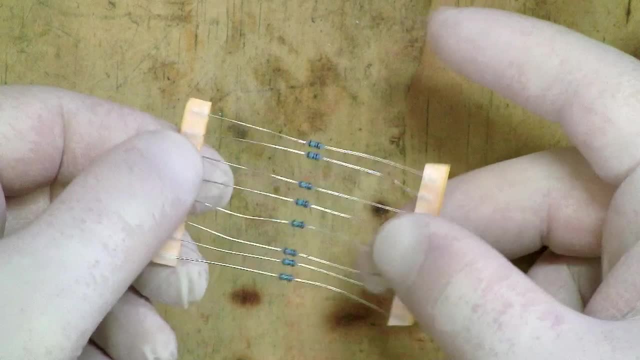 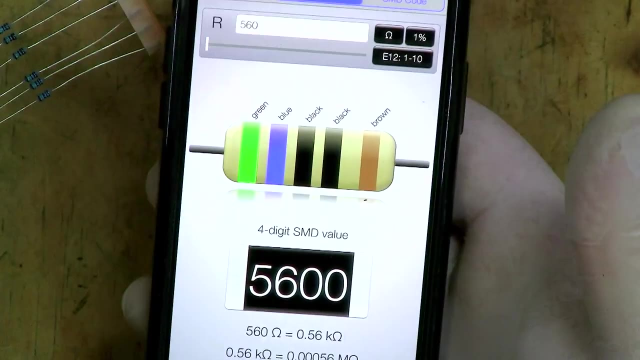 all of the colors and what they mean and how you figure out what the key, the resistance, is, based on those colors. I'm an extremely lazy person, so I actually just use this utility here, called resistor toolkit, on my phone. it allows me to just select what colors the bands are and then it'll. 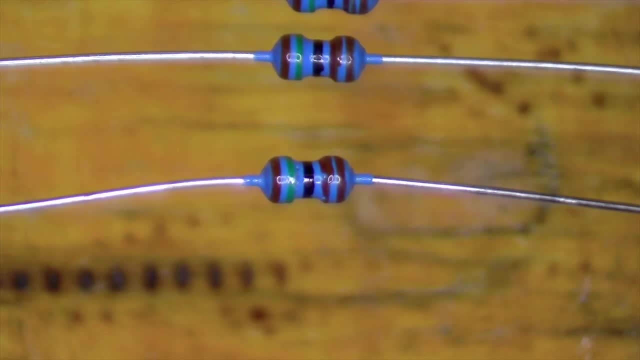 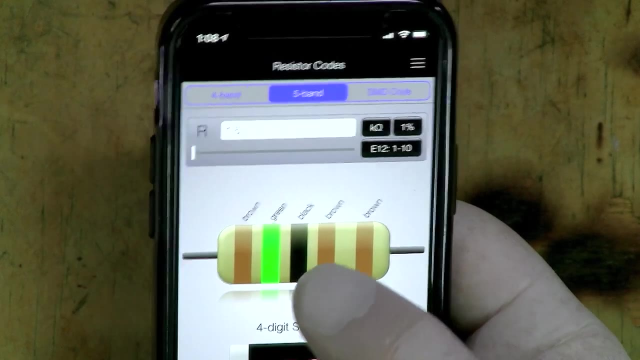 tell me what the resistance is. so looking at these resistors here under the microscope, we can see that they're all the same, so I'm going to put them in place. and then I'm going to put them in place that they're brown, green, black, brown brown. now, when I put that into my software, here it tells: 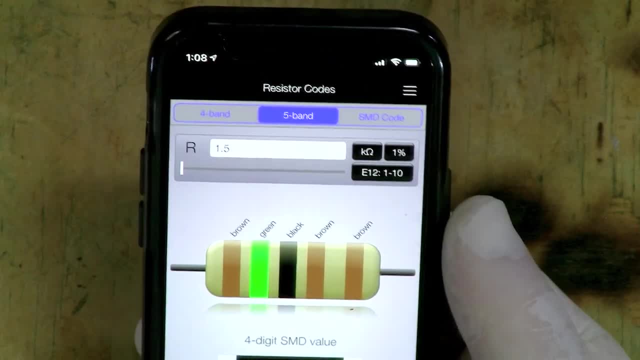 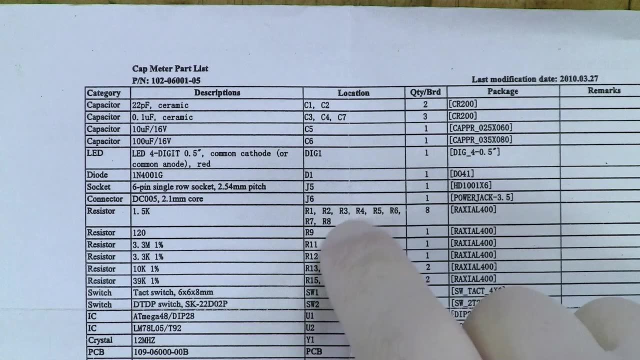 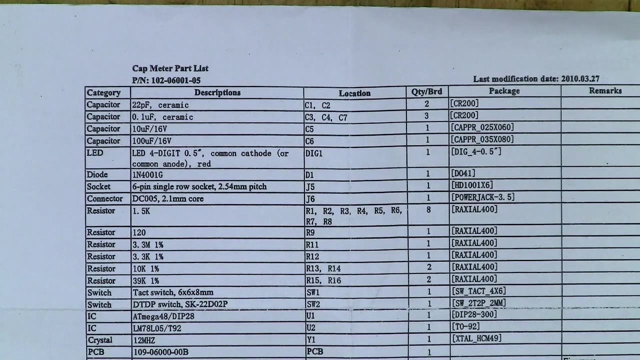 me that that is 1.5 kilo ohms. so if we have a look at our instructions we can see here resistor 1.5 K and that goes in positions R1, R2, R3, R4, R5, R6, R7 and R8. so let's put those into the board. 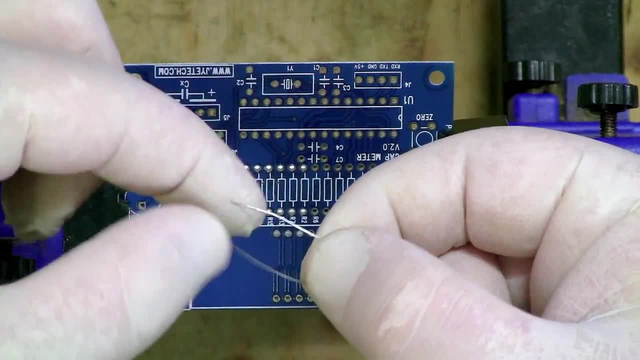 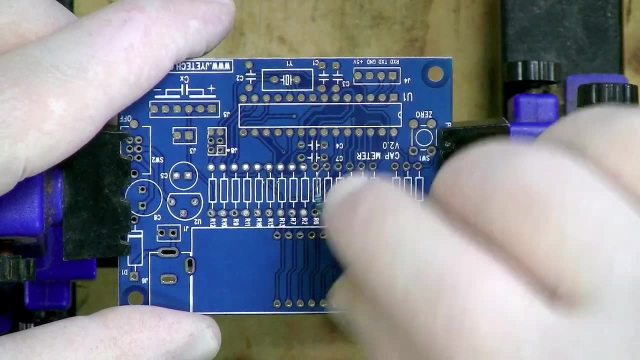 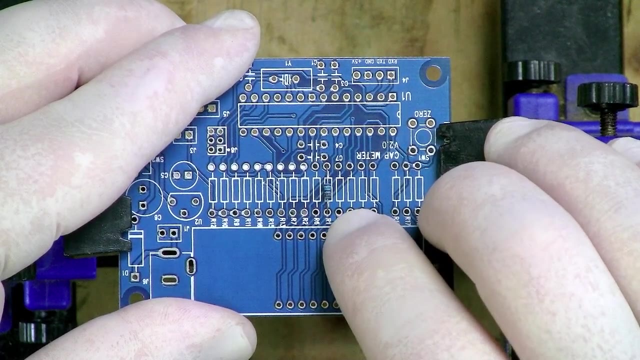 okay, so I'm going to get one of these resistors. I'm just going to bend the pins like that and then I'll feed it into R1 here. okay, now, this is a resistor. resistors aren't polarized, so it doesn't matter which way around. 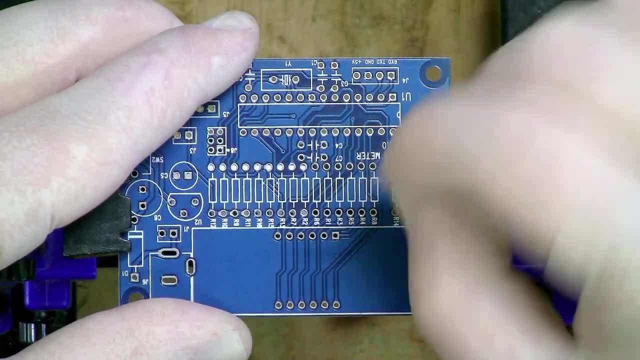 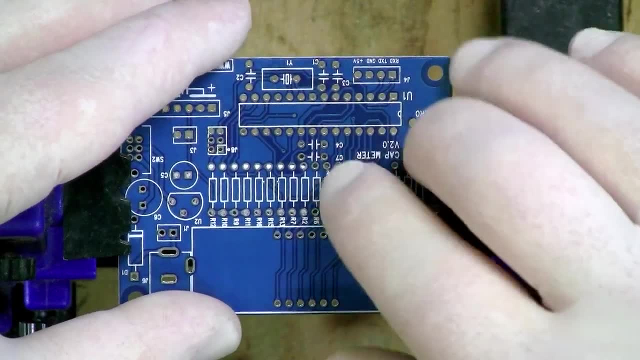 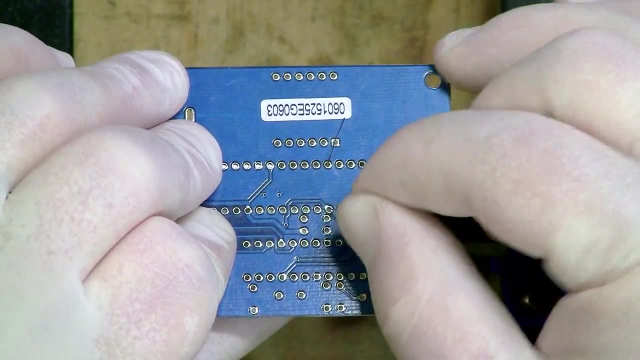 you put them, so I can put it in that way, or I can spin it around and put it in that way. okay, now, once it's in position here, I want to. I want to make sure it doesn't actually fall out when I spin this over, so what I do is I. 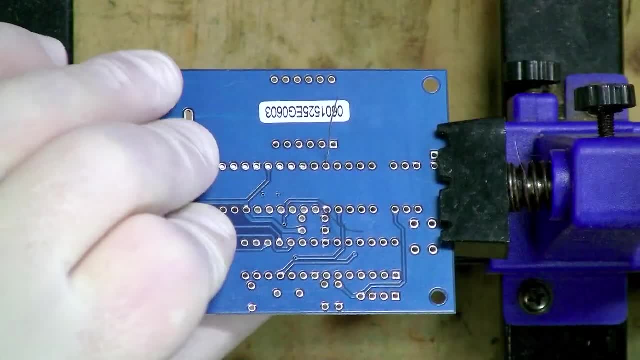 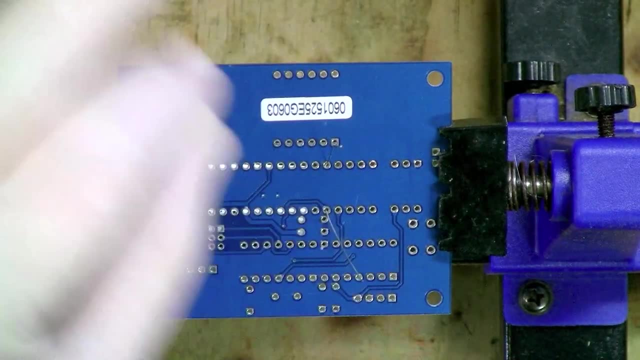 just grab these pins and I just bend them slightly. I don't bend them a whole lot, just enough to stop the component from actually falling off the board until I solder it. some people like to bend them all the way flat, but I prefer not to do that because I find that if you accidentally put the 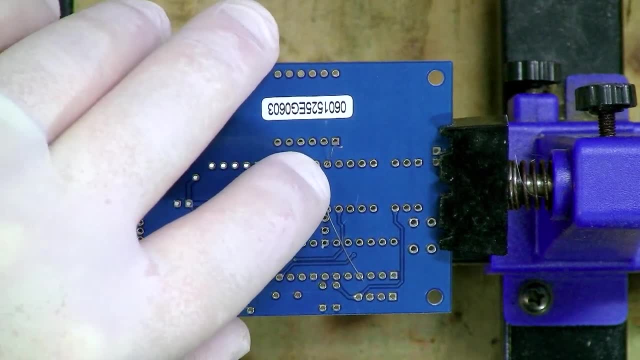 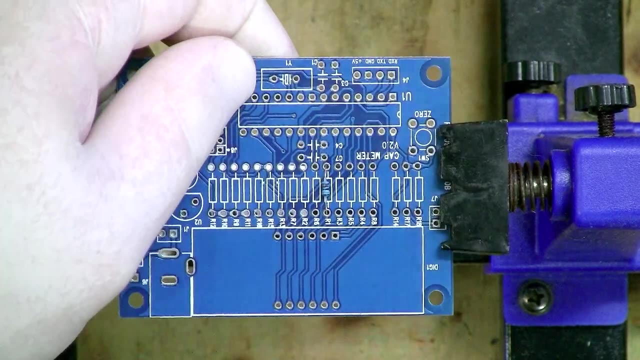 wrong component in the wrong place it's. it's a lot harder to desolder and remove that component if the pins are completely flat, so I just try and bend them, just the bare minimum to hold that component in place. right now I'm going to solder this in. 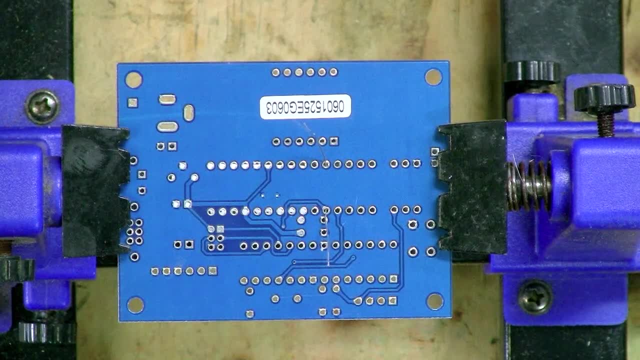 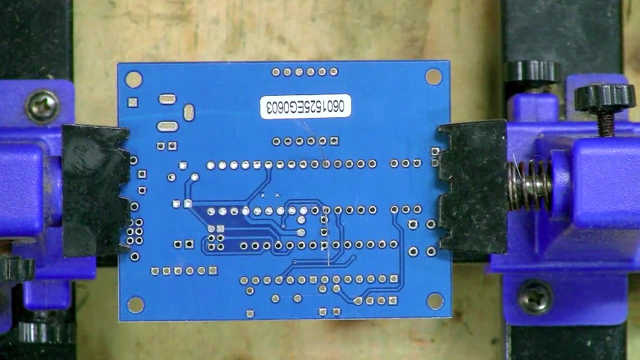 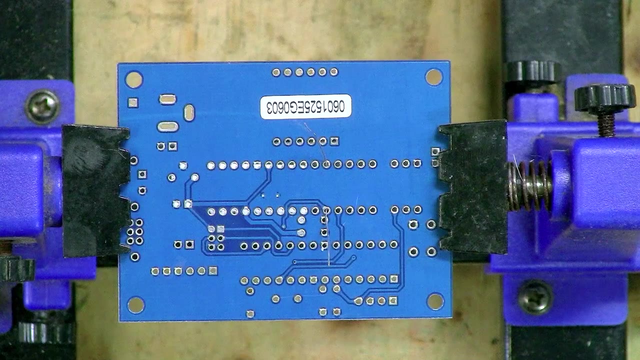 position. now I am using my budget soldering iron today. you will find links in the description for this one. an interesting thing: in my last video I used a very, very cheap soldering iron, and I have. I've actually had a lot of people come to me and say: where can I buy that soldering? 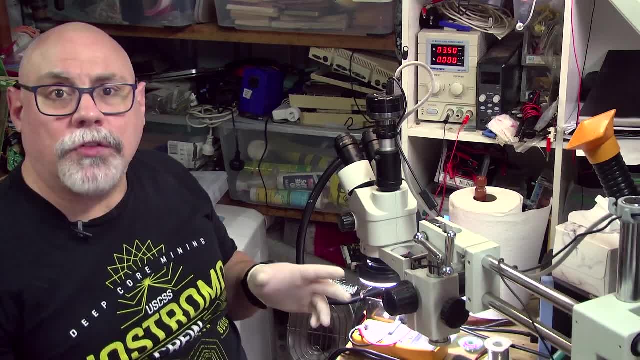 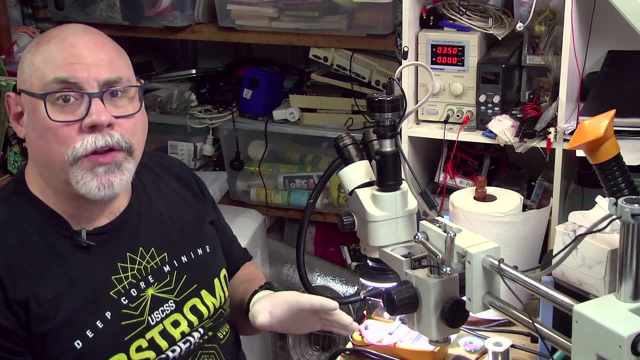 iron that you used in the video. now I used that soldering iron to demonstrate that soldering was more about technique than it was about equipment. however, that particular soldering on has some massive design flaws, so I wouldn't actually recommend that. I do have budget soldering. 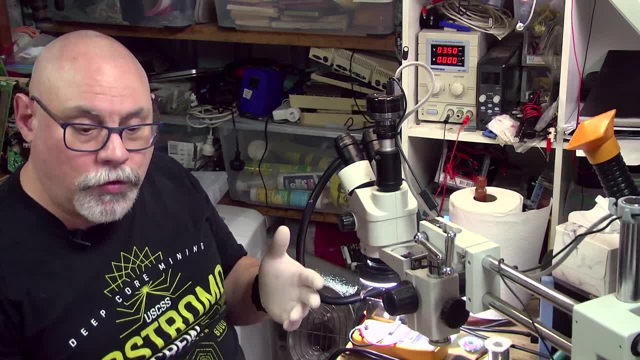 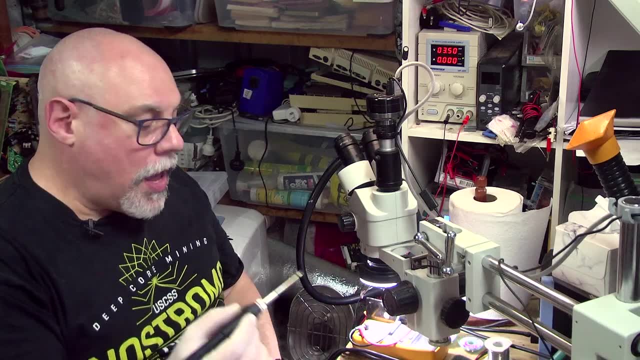 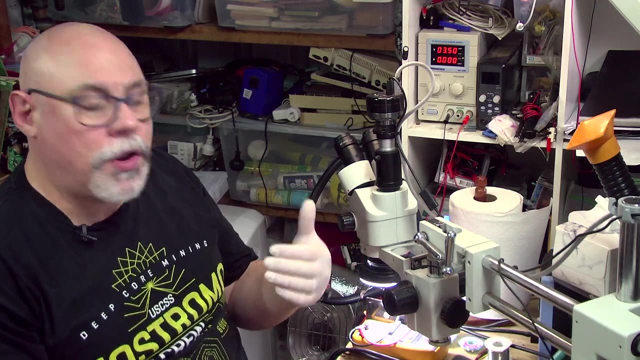 irons in the description that I recommend, if you want to, to use them. I'm actually using one today, um, for soldering, so this is one of the budget ones, and I'm also using a conical tip. now, I don't like using conical tips, I like to use bevel tips on my soldering iron. 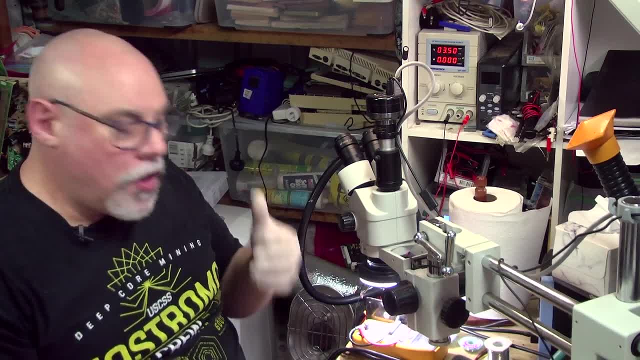 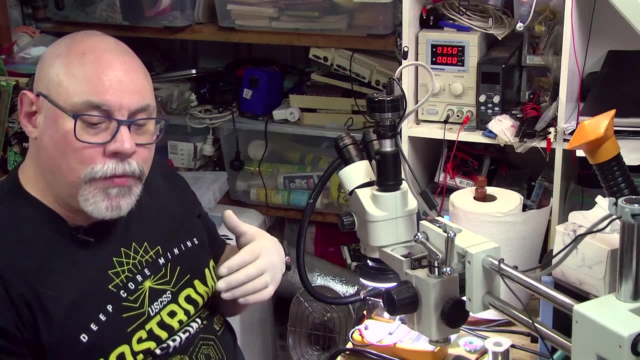 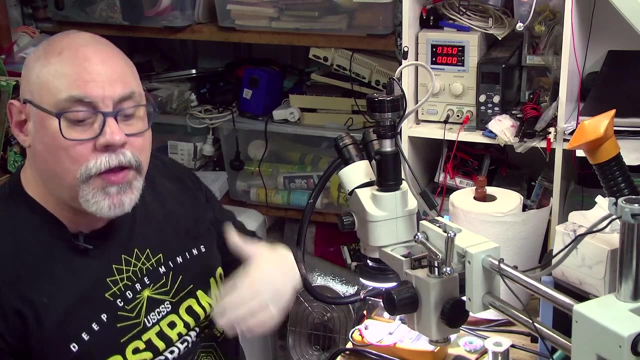 the most cheap soldering irons come with conical tips. I thought I would do this demonstration with a conical tip because that's what a lot of people will be using, so, um, I'm just going to give my tip a little bit of a clean. if you want information about the maintenance of the tips, please feel. 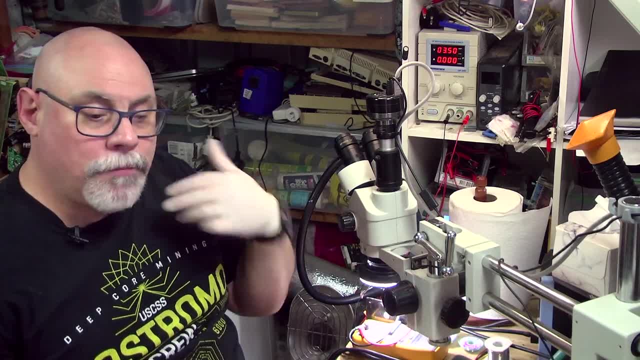 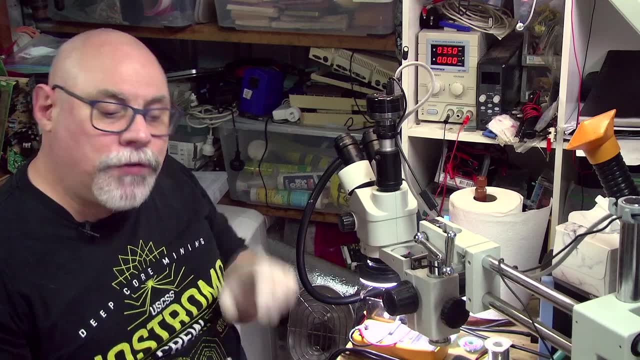 free to have a look at my beginner's guide to soldering video. I go into a lot of detail about that sort of stuff. one thing I do want to mention is someone did say: uh, if you're not using a soldering iron for a long period of time, an extended period of time- uh, leave it with a. 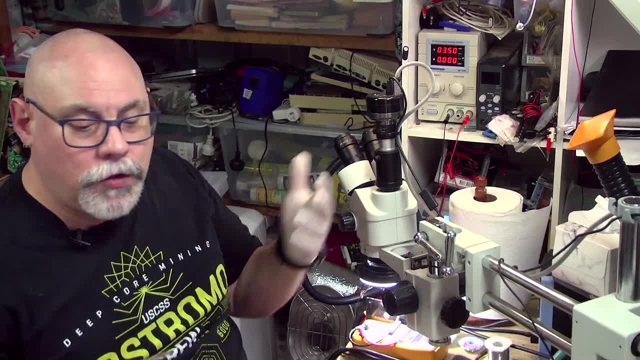 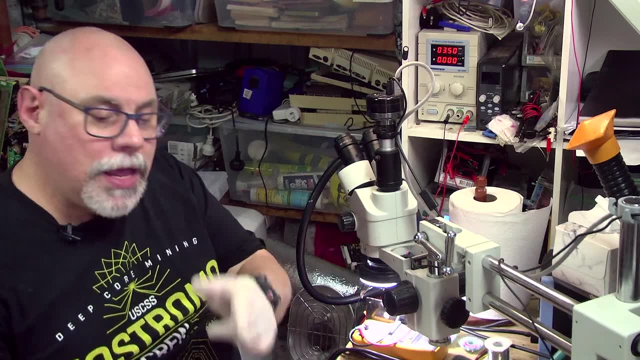 little bit of solder on the tip and that is a good one. I um, I tend to use my soldering on every day so I tend not to worry about that too much. but if you are someone who does a bit of soldering and then puts a soldering iron away, leave it with some solder on the tip. it will make that tip last. 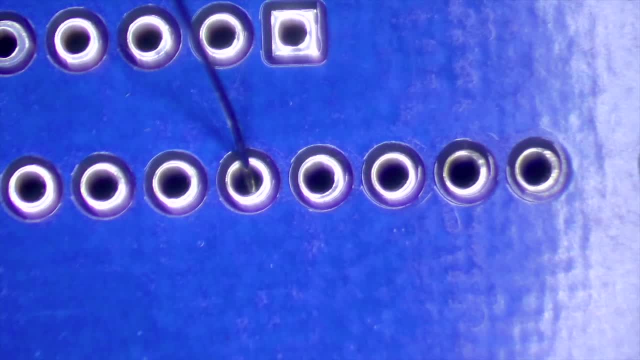 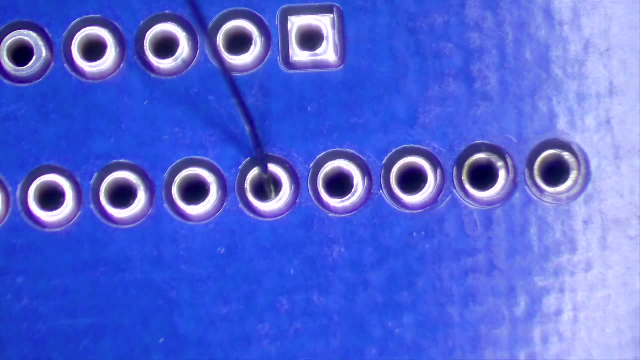 longer. okay, I'm going to use the- uh, the microscope view for this, uh, for this little bit, uh. the reason for that is I want you to be able to see the solder melting and hardening when I do this joint. so most important thing when you're soldering is you want to make sure that you are. 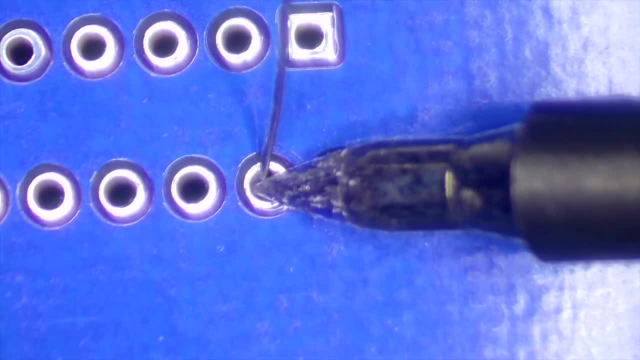 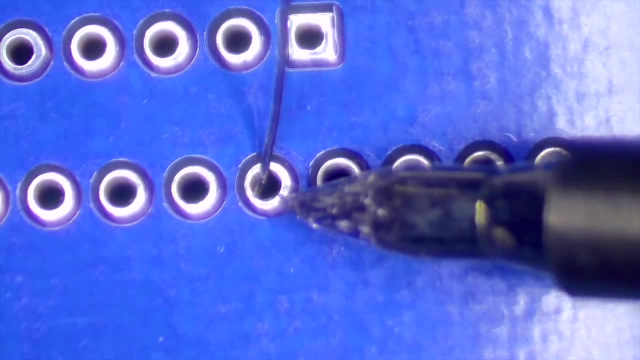 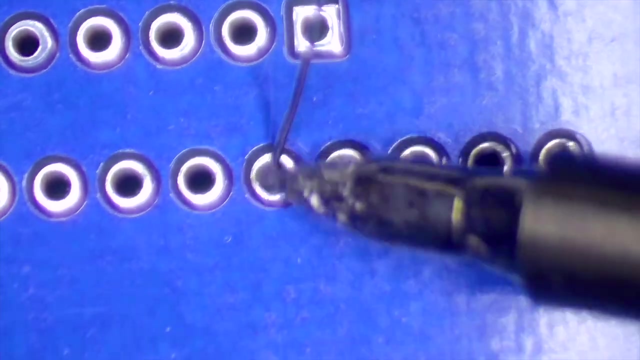 getting everything that you want to solder nice and hot. you don't put the solder onto the tip and then the tip and then try and transfer the solder onto what you're soldering you want to melt. you want to get these, the things you're soldering, hot and then melt the solder onto it, okay, so. 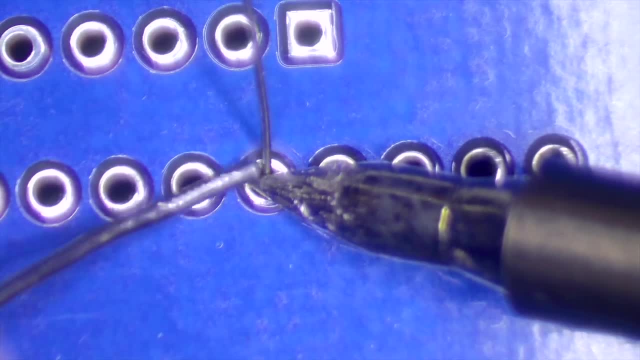 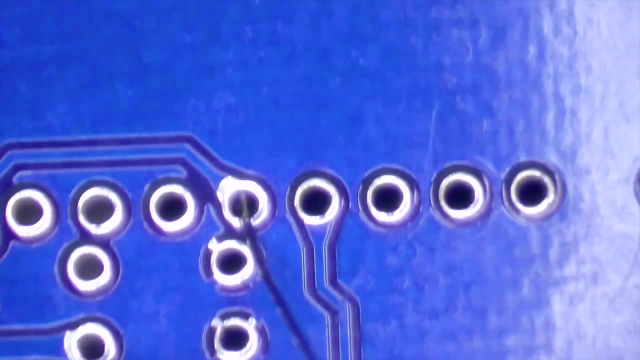 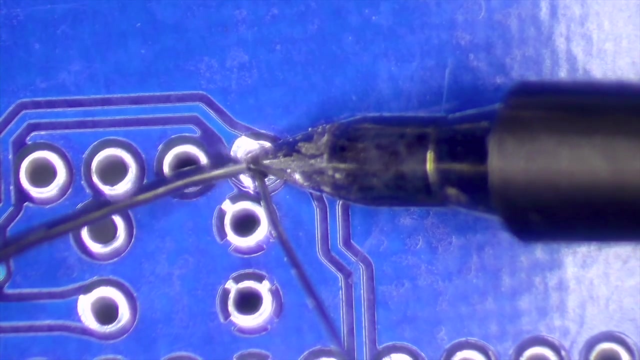 let's get that hot and we put some solder on it and we will melt that onto the tip there and then you can see it as it hardens there. let's go on to this next one. let's get them nice and hot, melt the solder onto the tip, that's onto the components, transfers onto there and, as you can, 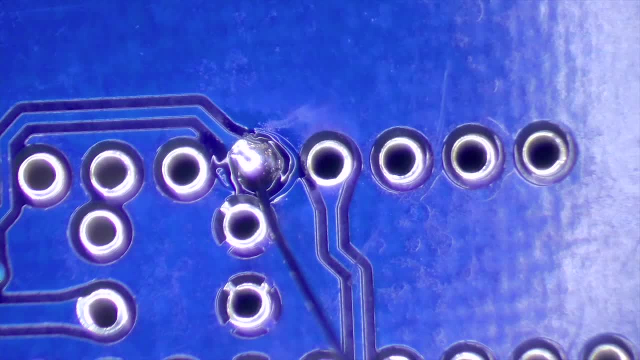 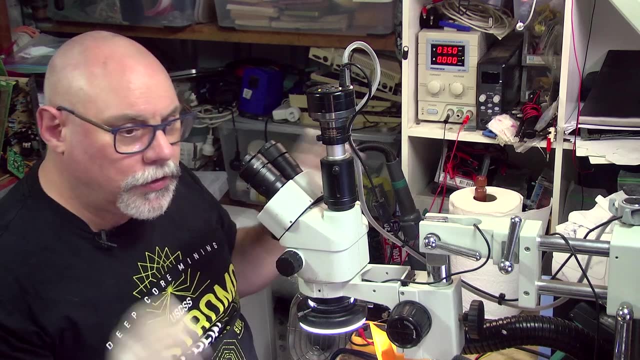 see, there's a lovely joint there, nice and neat and tidy. we don't have too much solder, we don't have too little, and when you see the smoke coming off that there, I've had a few people that have put comments in the video saying: oh you know, this is lead, this is bad, it's dangerous to breathe in. 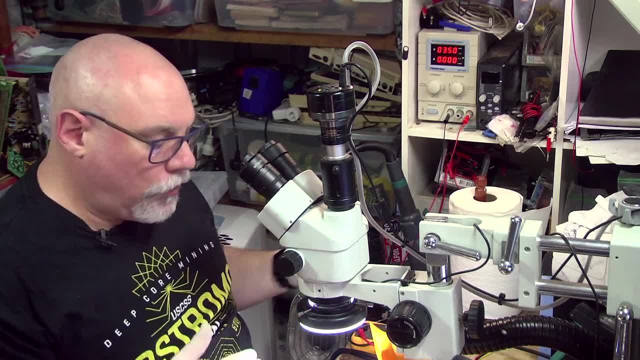 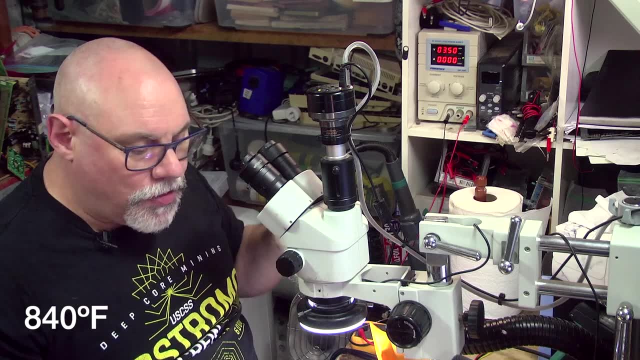 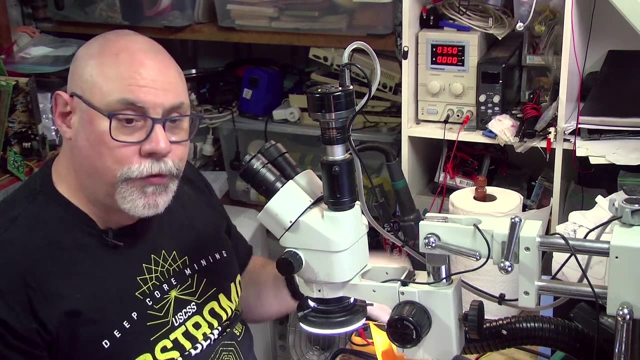 it's not lead lead. it doesn't go gaseous at this sort of temperature. it takes temperatures over 450 C for lead to for you end up with lead gases. however, that what you're seeing with the smoke is you're seeing flux burning off. now. that's not good for you, so you need to make sure that you've got some fume. 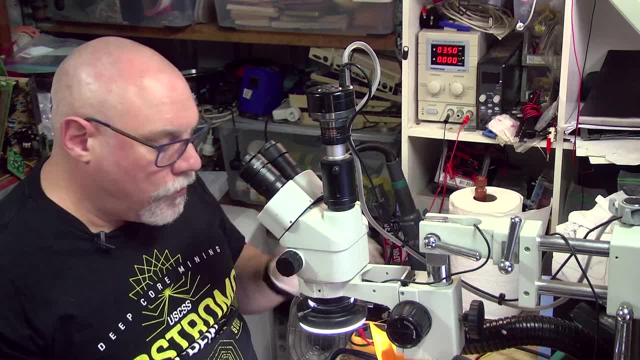 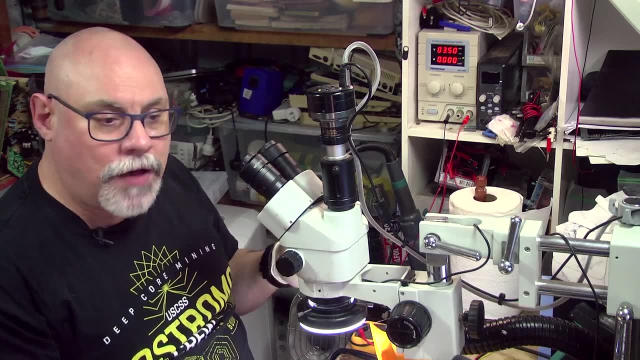 extraction, or you've got a fan set up or you know you're very well ventilated area. when you are working with lead, though, it is very important to have gloves or to wash your hands thoroughly afterwards, because if you're working with leaded solder, you don't want. 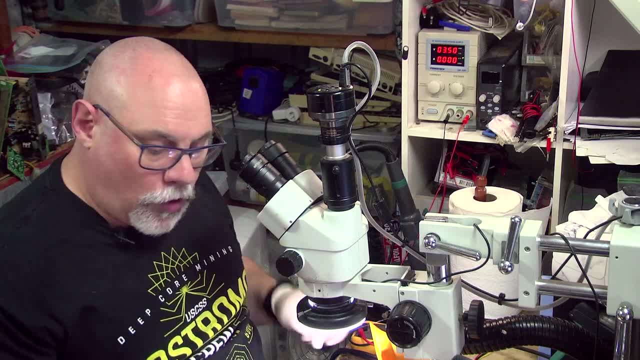 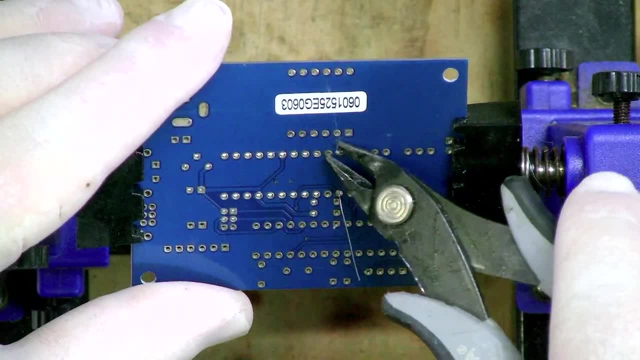 to transfer that lead to your mouth or to your eyes. so so I am using leaded solder. I prefer to use leaded solder. okay, now we want to clip off the excess of those pins, so I'm just going to grab my little side cutters here and just give that a little snip. and give that a little snip and that's. 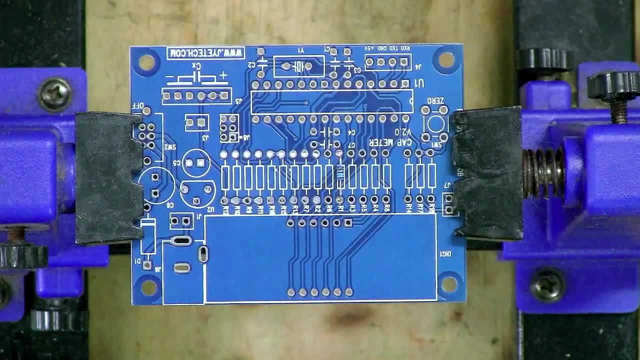 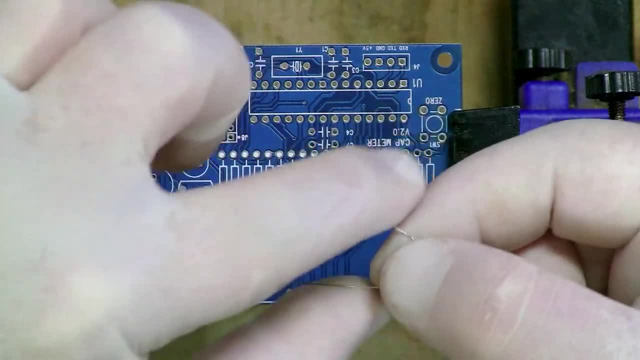 one component all soldered into place. let's do one more, and so it's the same. I get the resistor. I'm going to just bend those pins, I'm going to put him where he needs to be, and this one is in R2, so we'll just pop that in there.